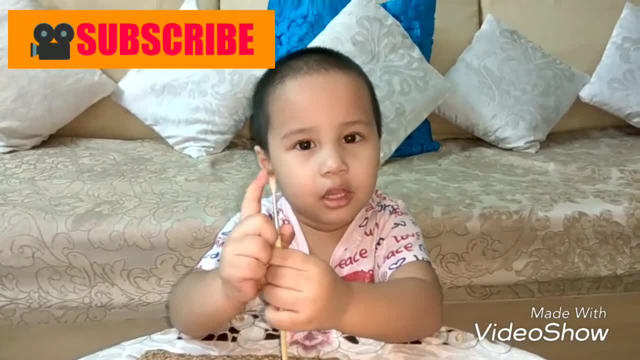 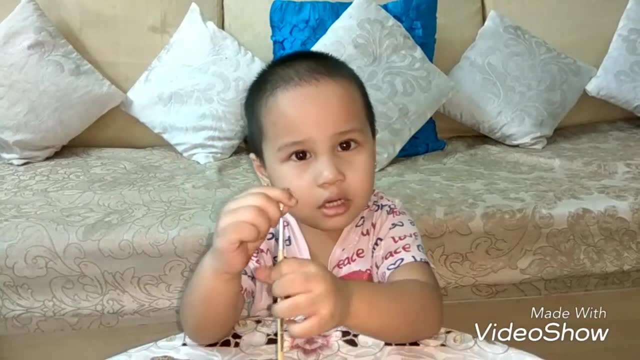 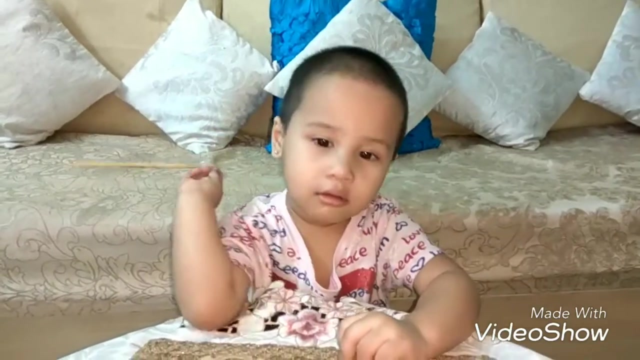 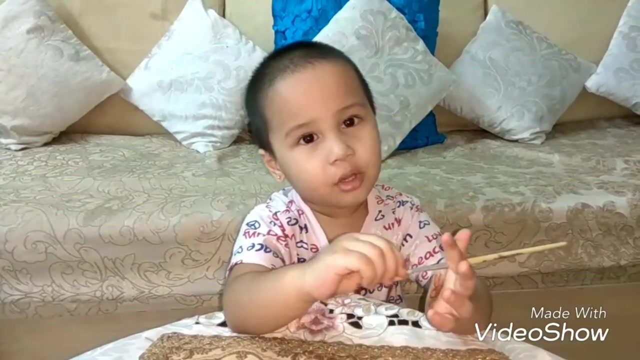 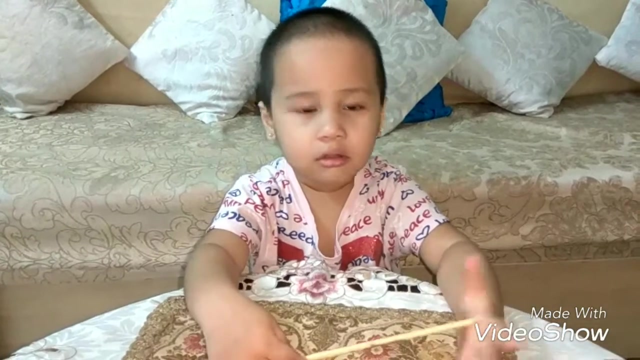 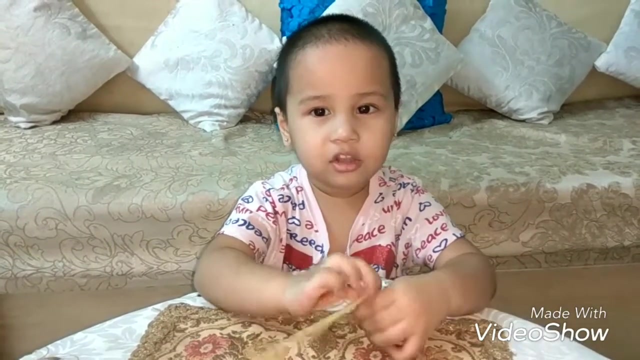 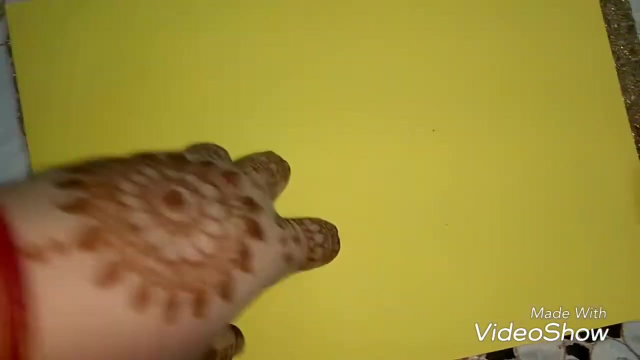 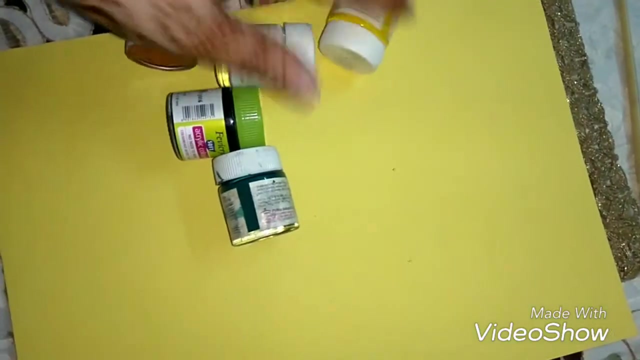 Hi, how are you? Hi, how are you? So, today I am going to make my art crowd. Let's get started. Go, do you like my video Sheet? then some colors, lots of colors. Pencil and water. 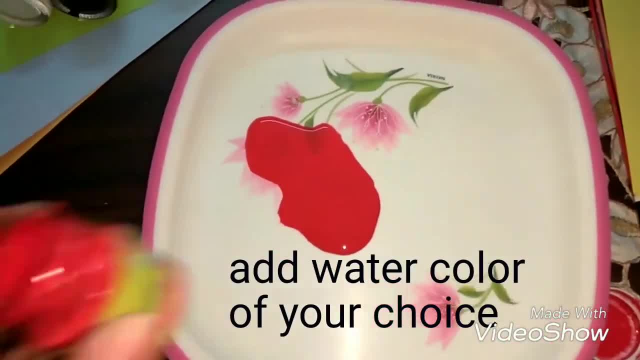 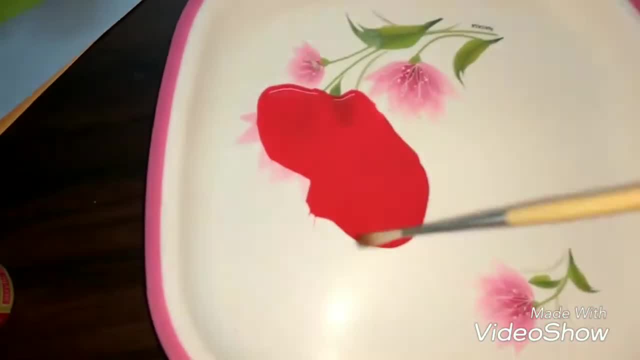 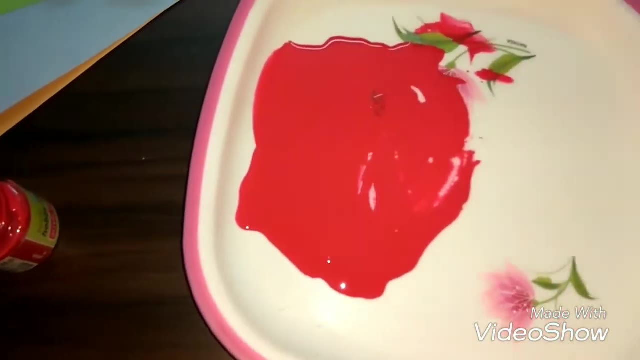 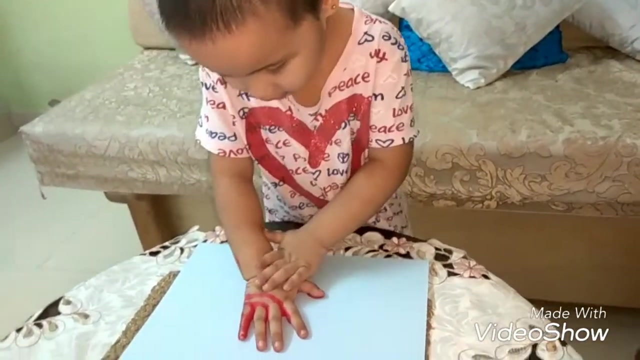 OK, Okay, Body roll, baby. Okay, Okay, Two, one, two go. Two, one, two go. Keep empty space and lots of blue for the three, but not black below. Ellulove, Ellulove, Ellulove. Ellulove, Elluloveolove, Ellulove, Risealtula, Ellulove, Ellulove, Ellulove, Ellulove, Ellulove, Ellulove, Ellulove, Rollulove Ellulove. 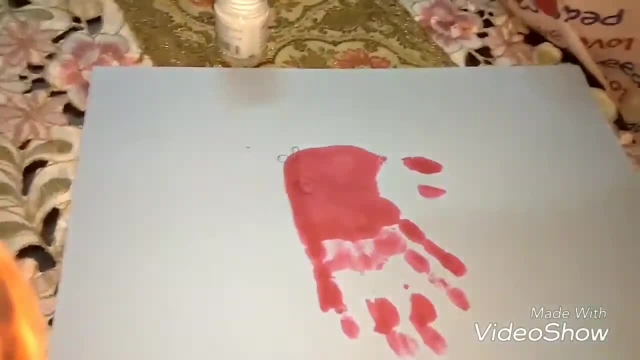 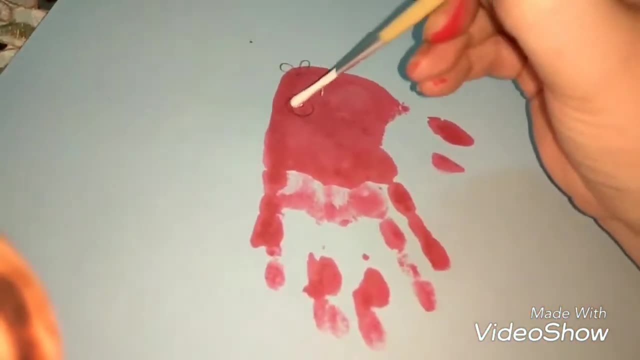 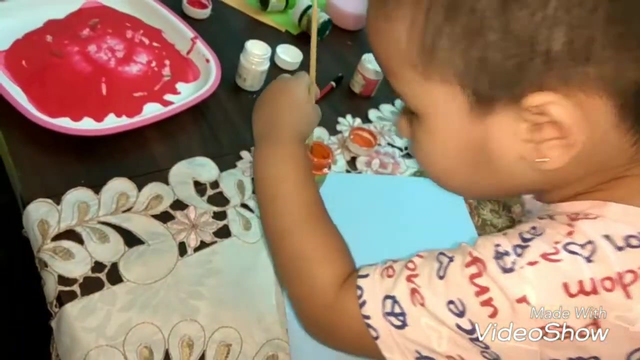 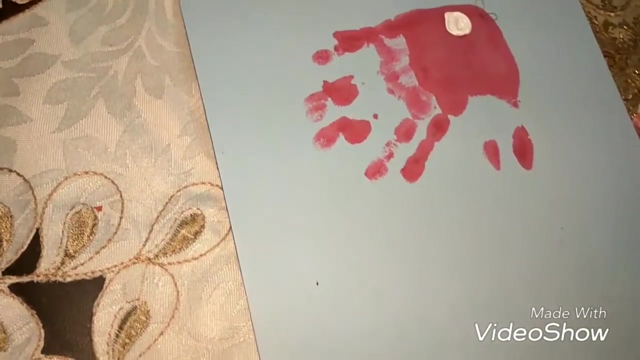 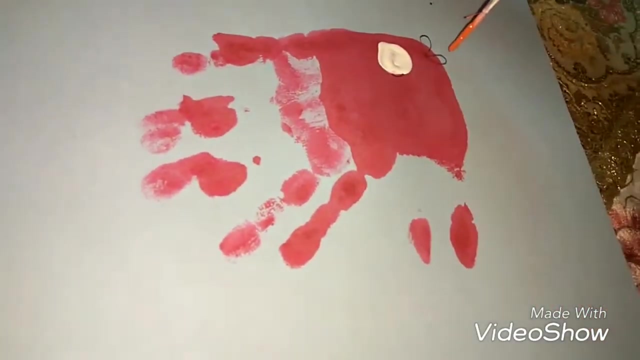 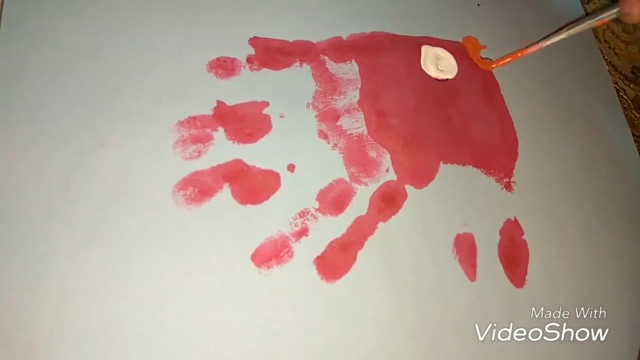 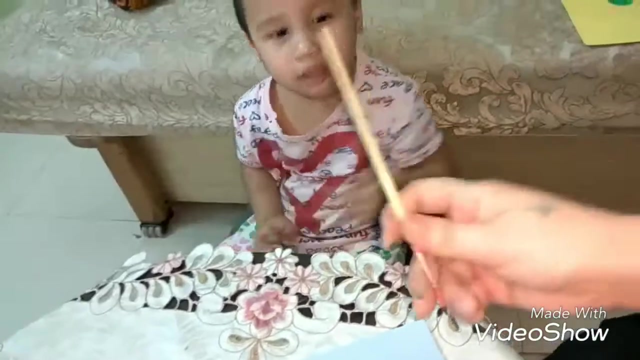 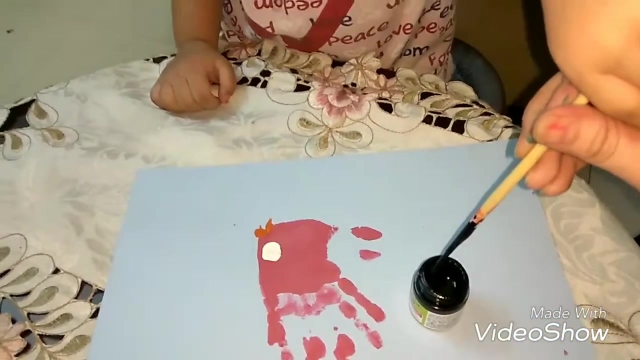 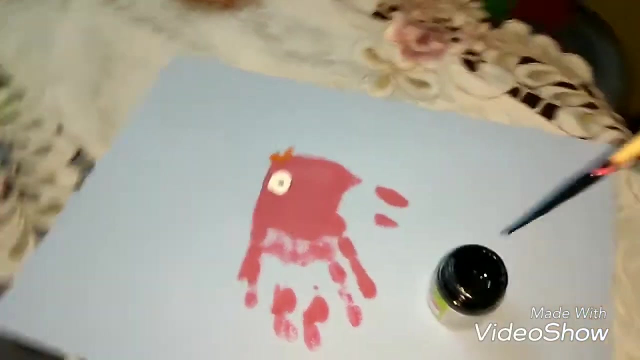 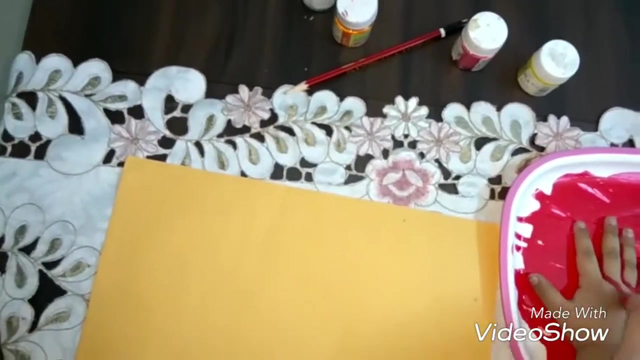 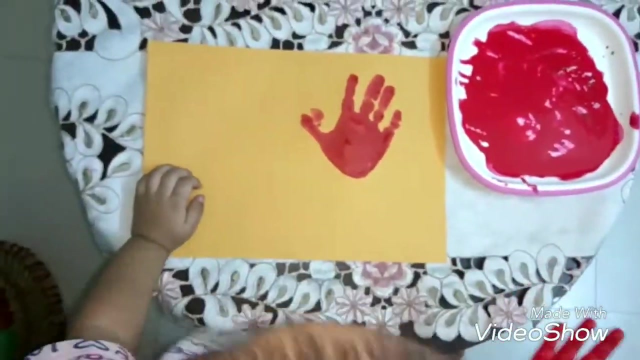 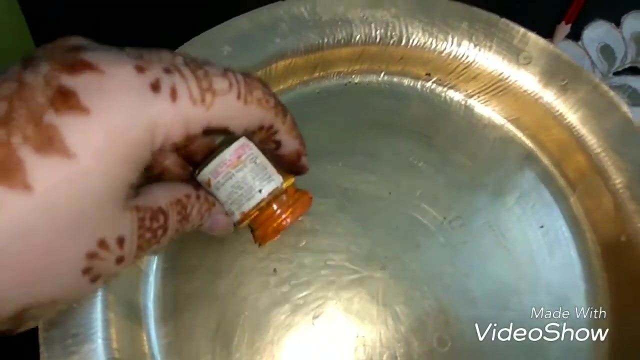 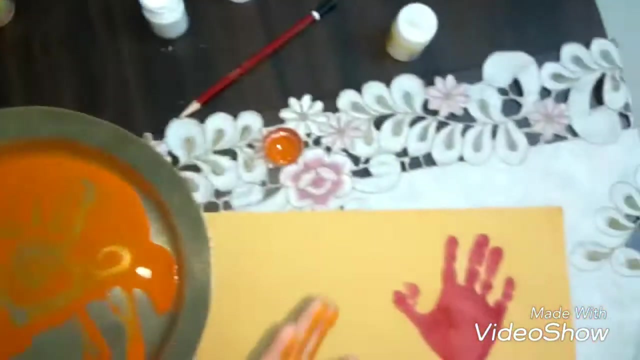 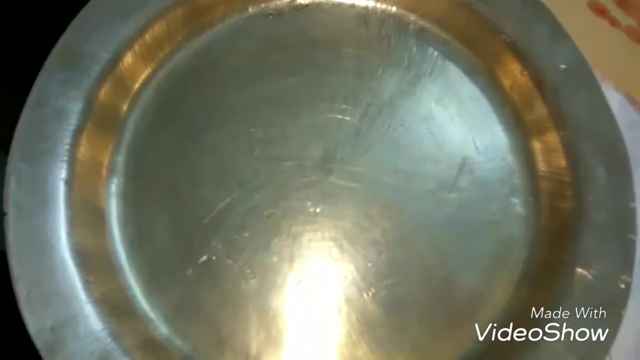 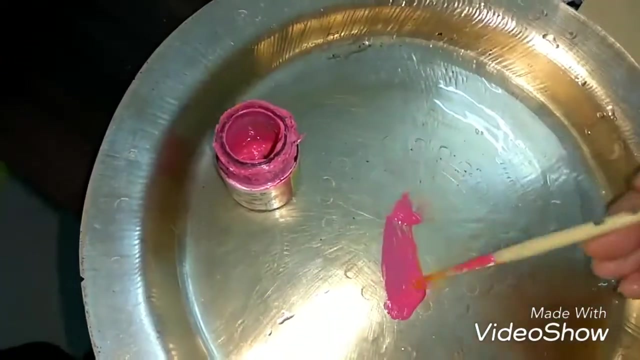 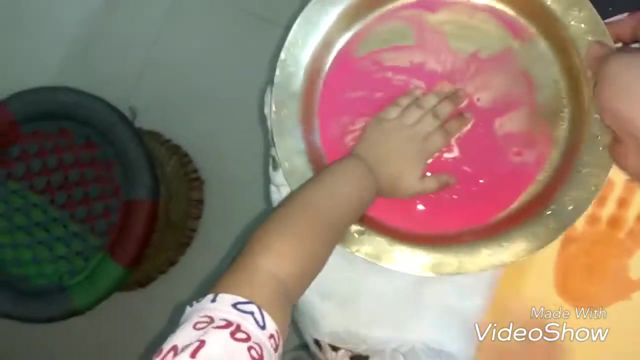 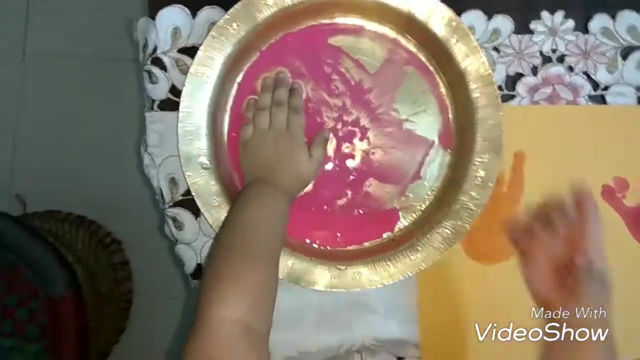 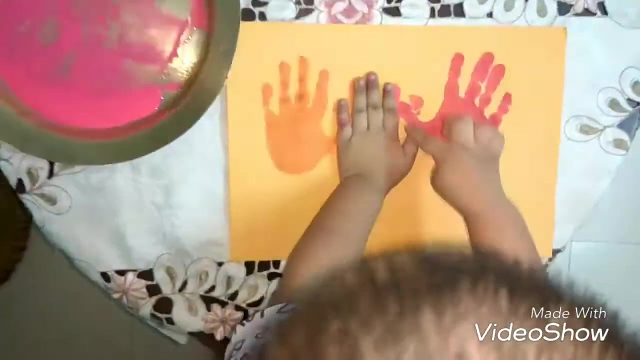 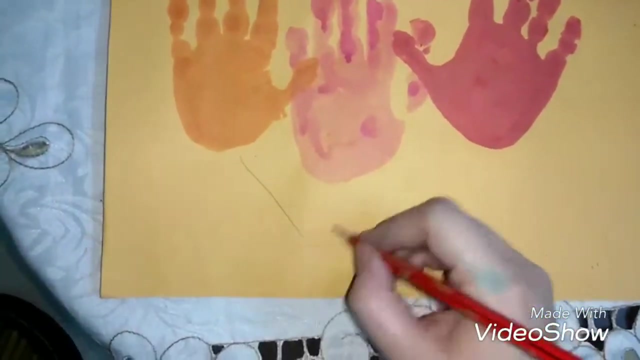 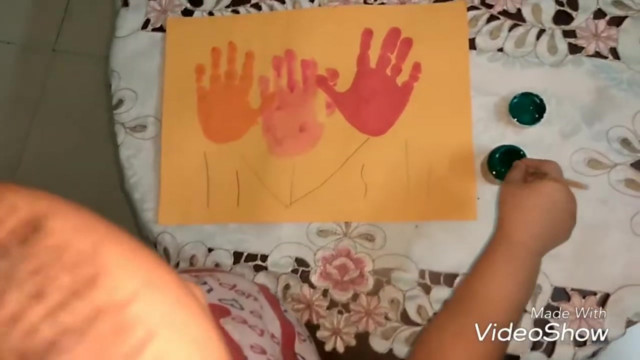 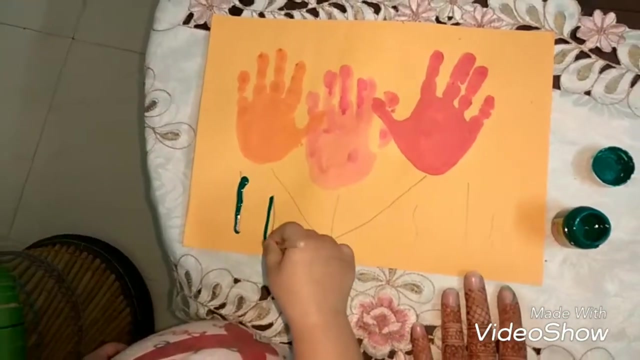 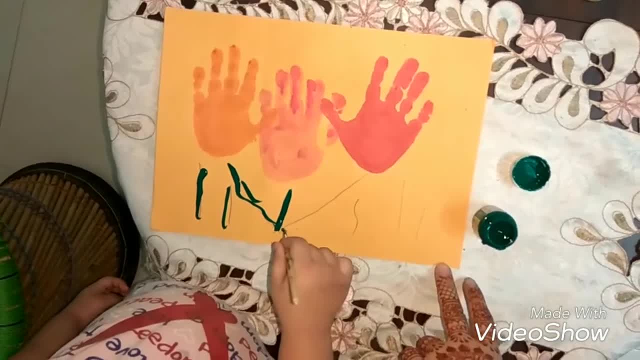 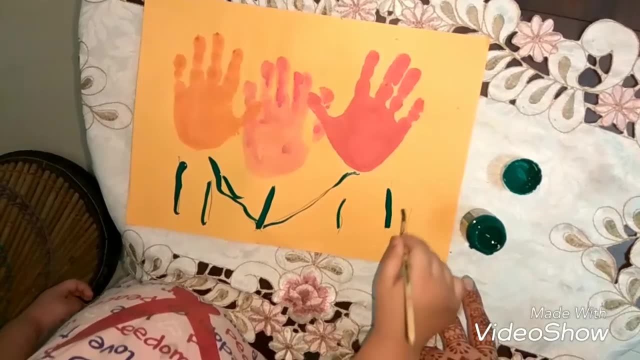 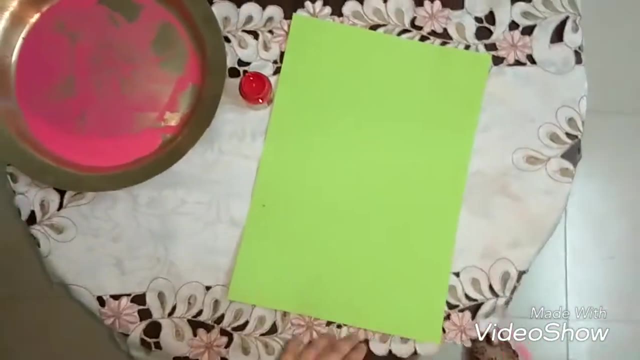 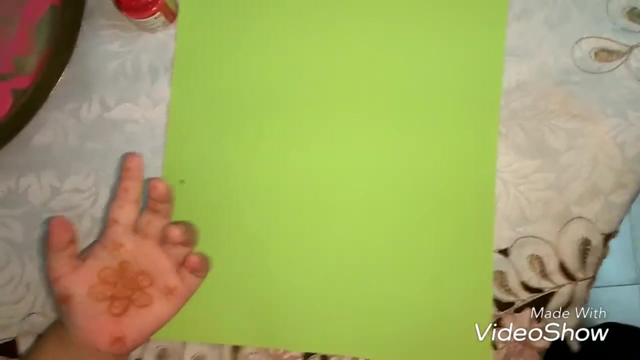 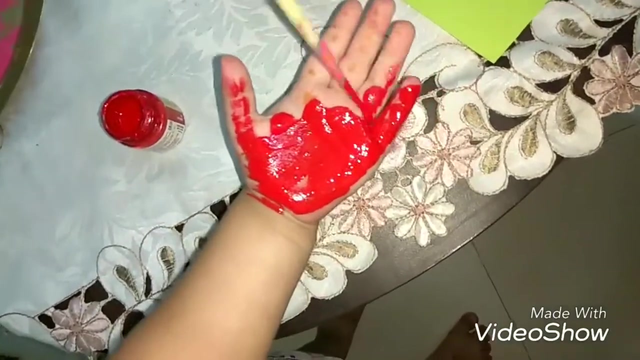 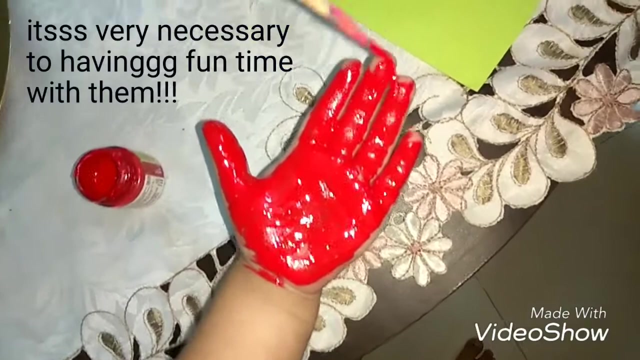 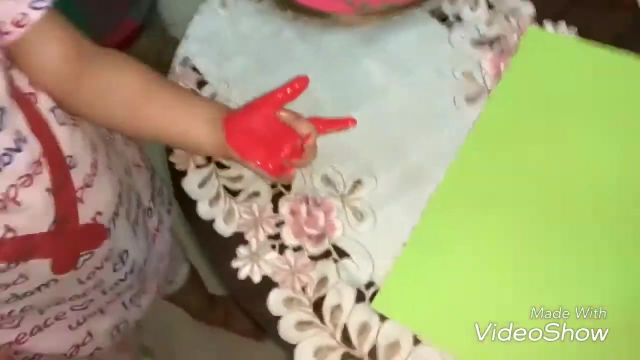 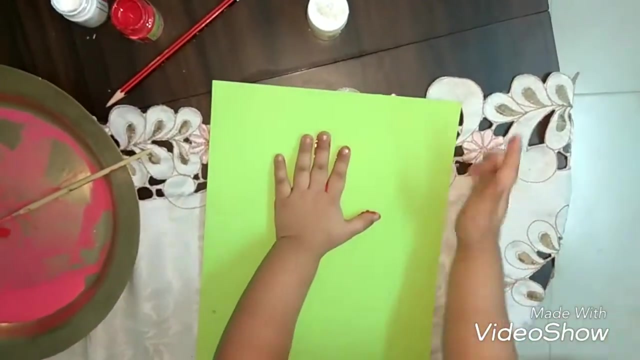 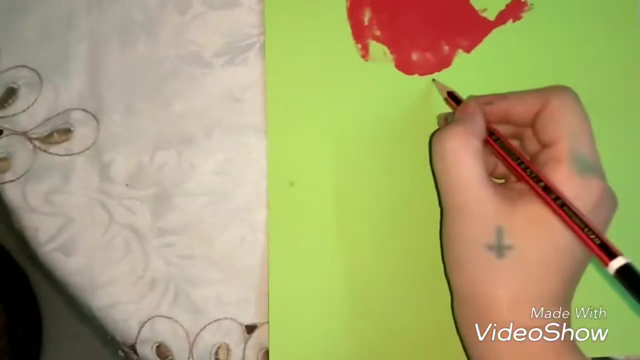 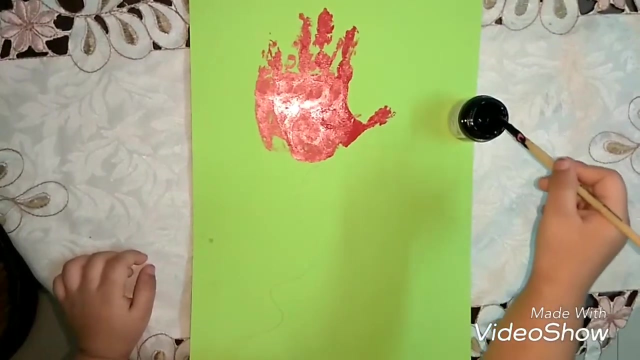 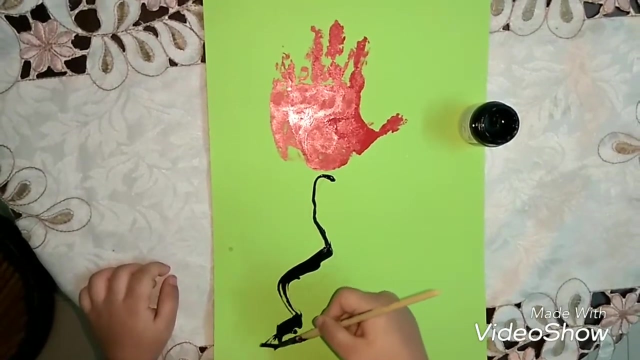 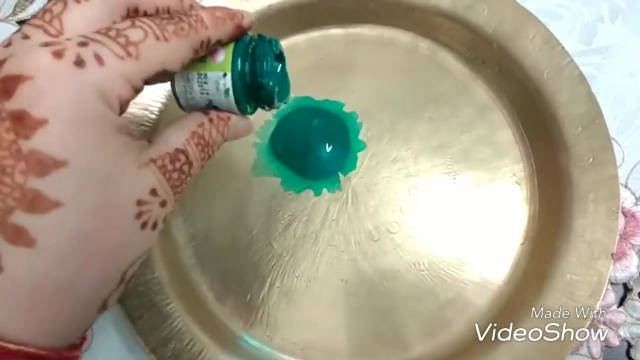 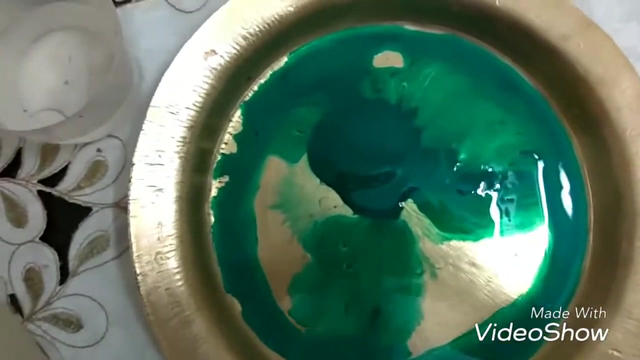 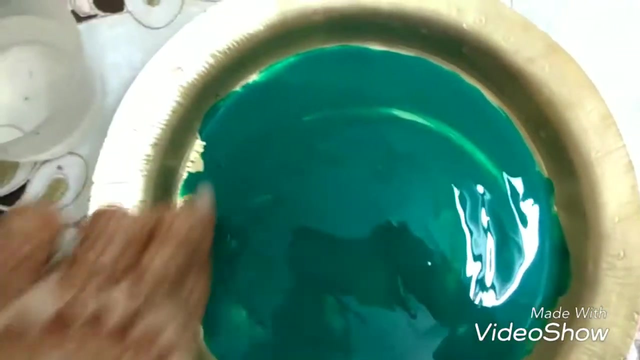 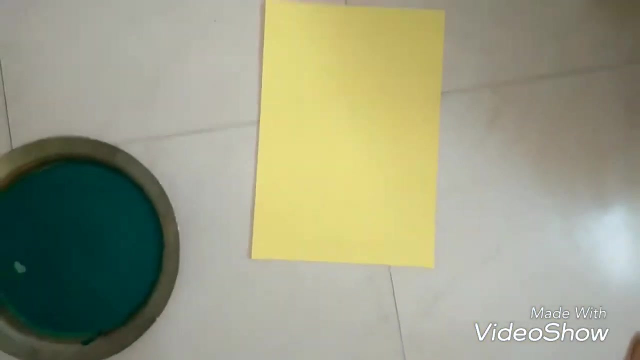 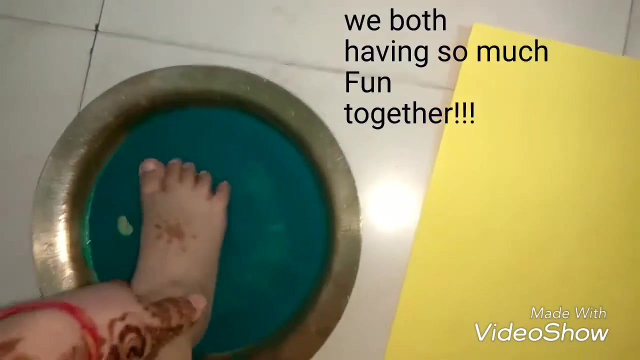 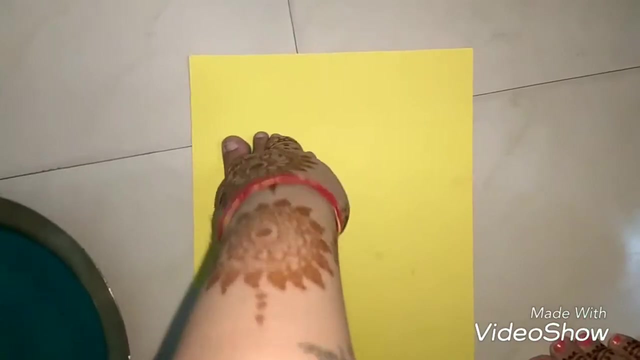 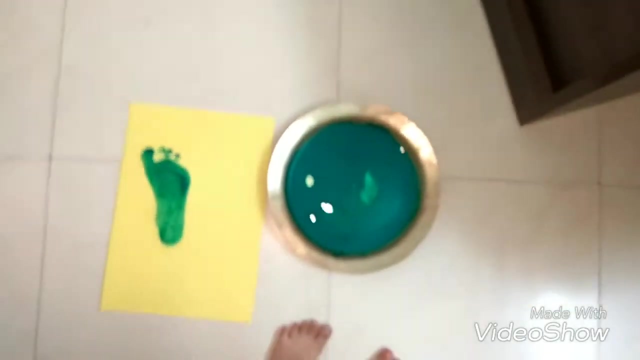 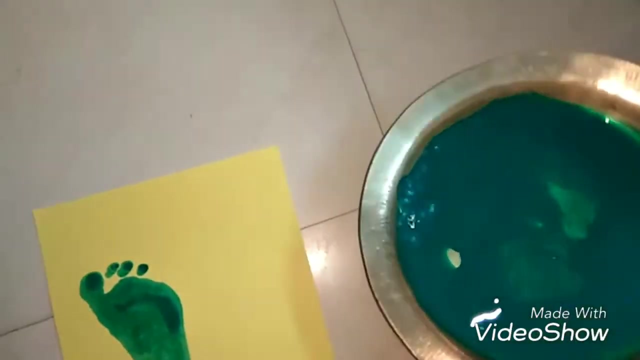 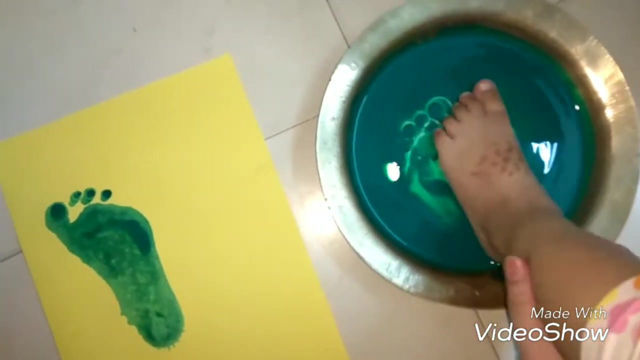 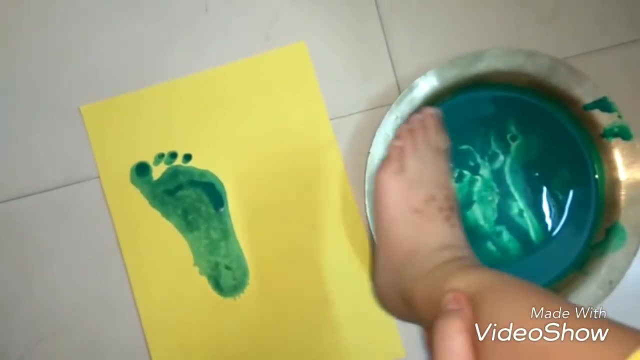 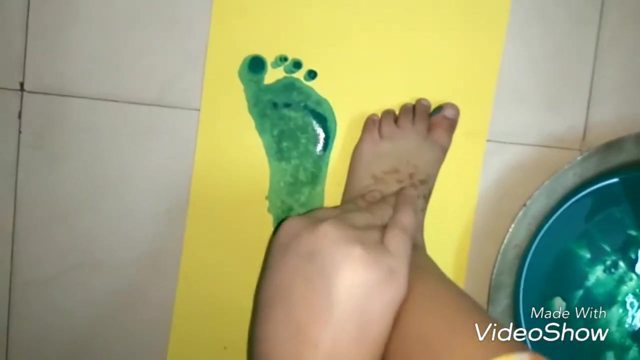 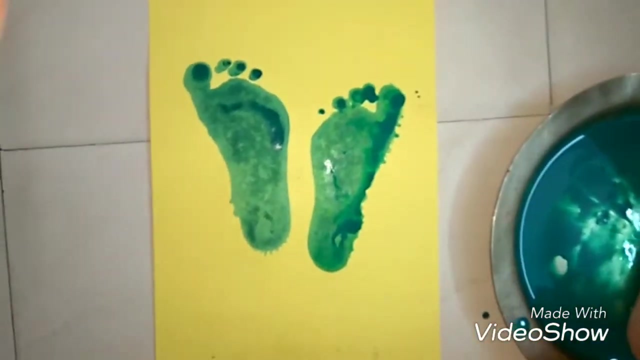 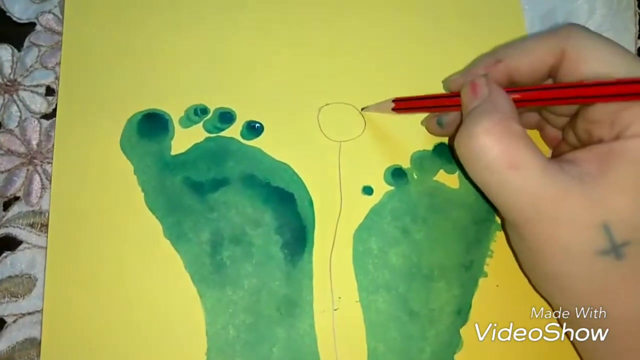 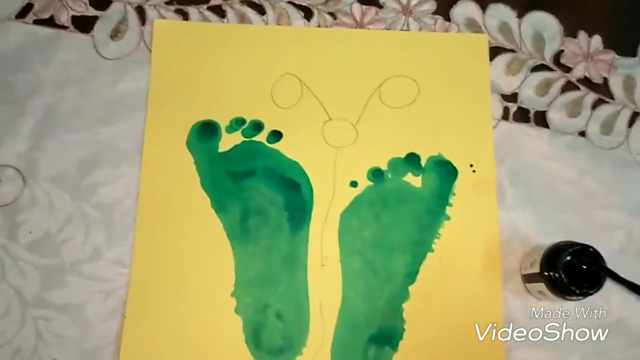 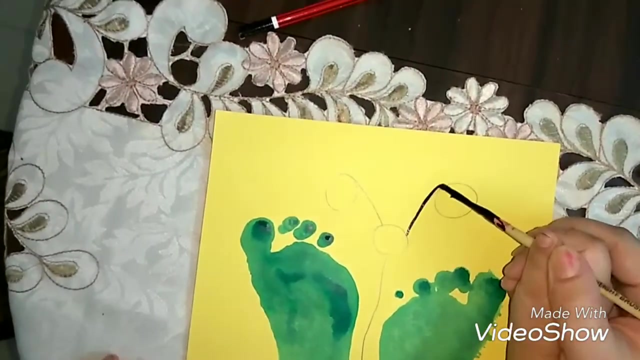 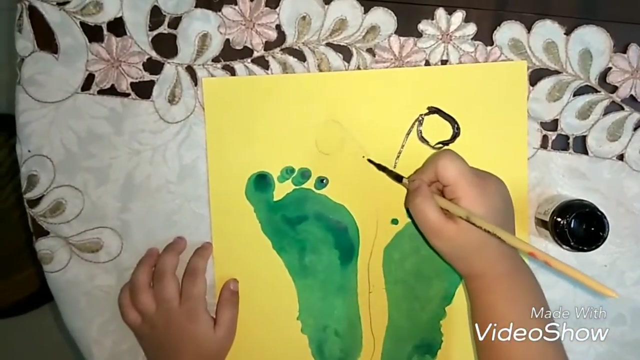 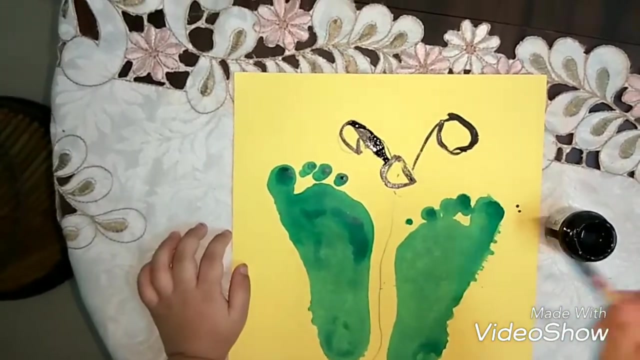 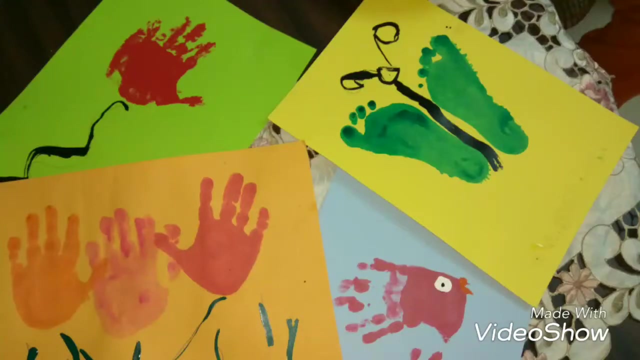 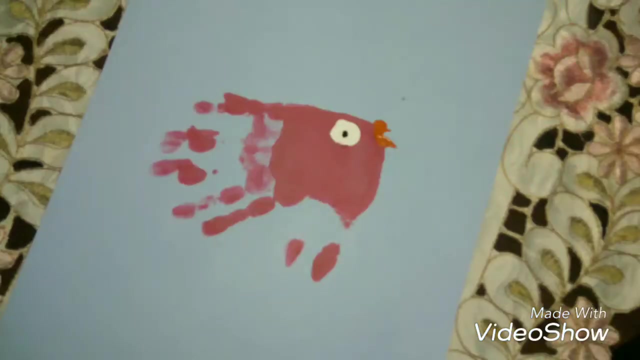 I am going to show you how to do it. And now another sheet. And now another sheet, And now another sheet. We'll see you next time. Bye-bye, Bye-bye, Bye-bye, Bye-bye, Bye-bye. Bye-bye.